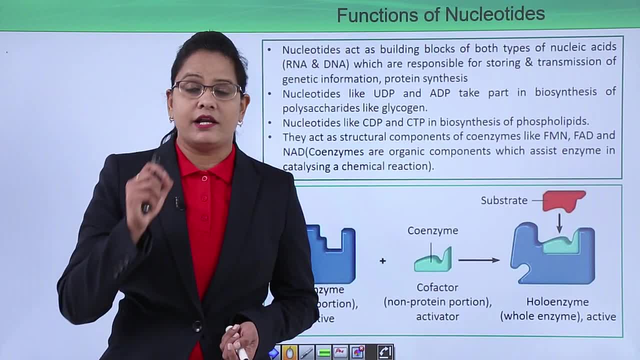 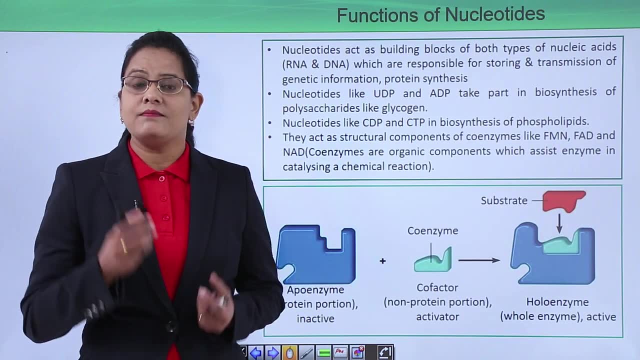 They help in biosynthesis of phospholipids. Now, another very important role of nucleotide is to act as coenzymes. Now what is a coenzyme? Coenzyme is a helper of enzyme. So enzymes sometimes on its own are inactive. 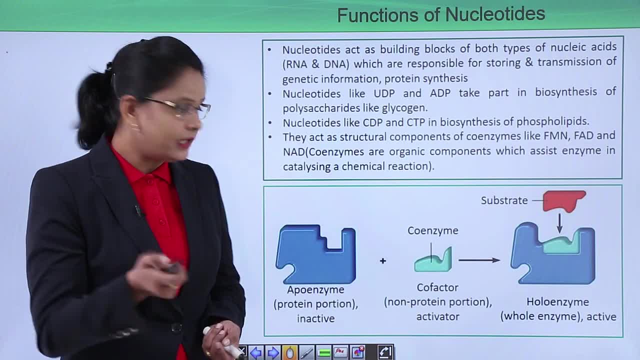 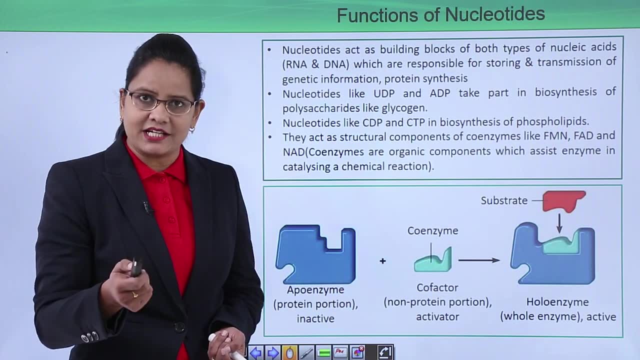 So they are known as apoenzymes or inactive enzyme. They, when combined with a coenzyme or a cofactor, makes it active, So after they have been activated, they are called holoenzymes. These holoenzymes can bind with the substrate and lead to a chemical reaction. 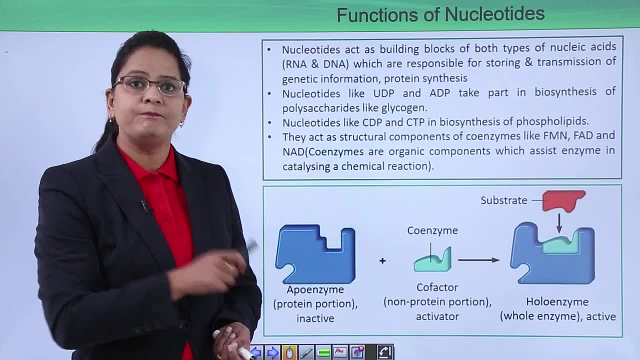 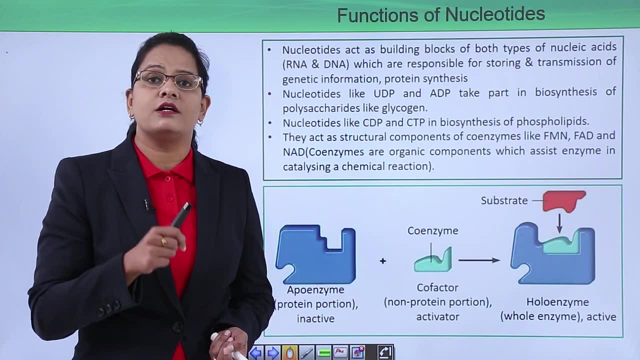 So the coenzymes are flavin adenine dinucleotide, flavin mononucleotide and nicotinamide adenine dinucleotide. So these are also. they are precursors for vitamin synthesis and they also act as coenzymes. 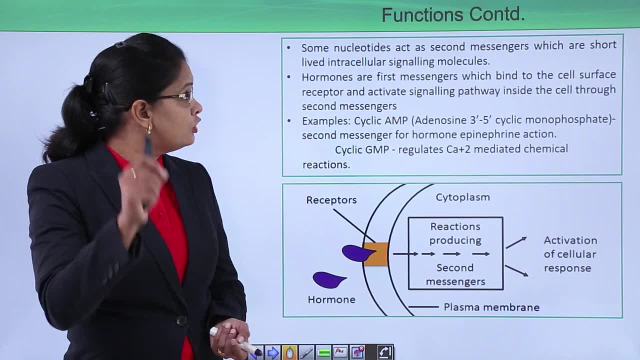 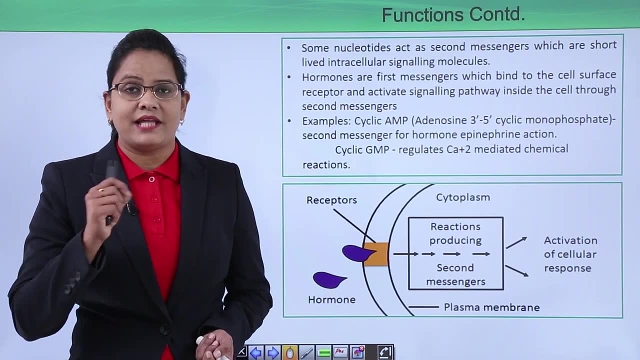 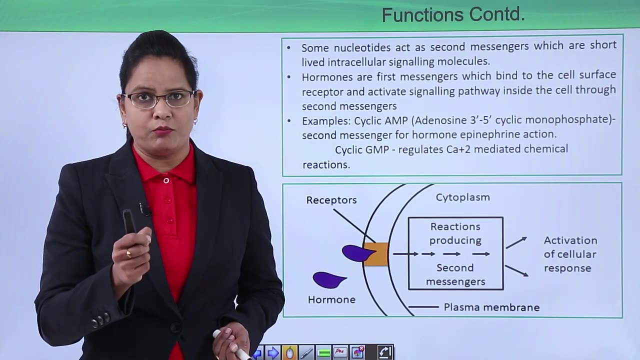 Now, another important function of a nucleotide is that signaling molecule. So these nucleotides, they act as second messengers, which means that they are intracellular signaling molecules. So when a first messenger, for example hormone in a cell, when a first messenger like hormone, 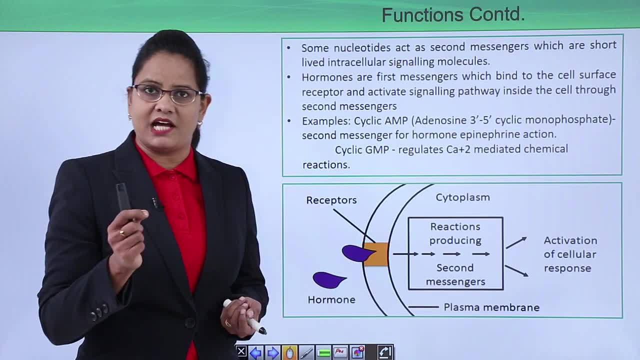 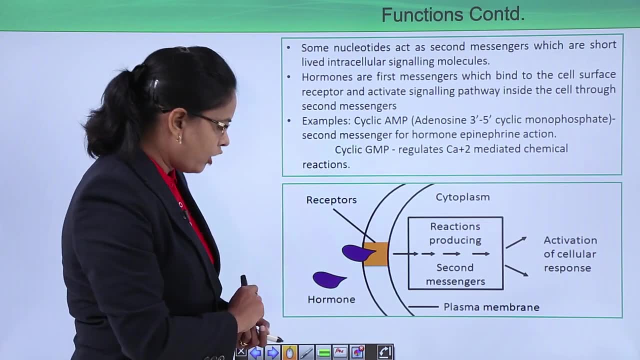 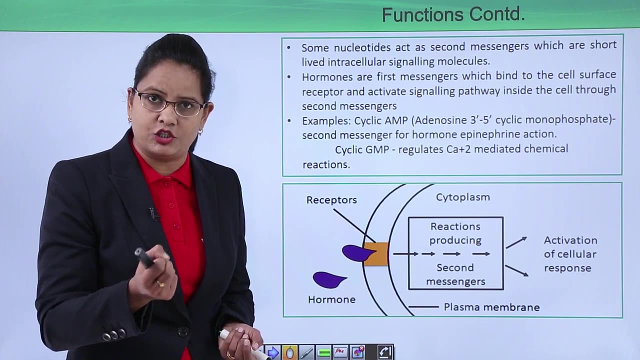 binds to the plasma membrane. there are receptors on the plasma membrane. We have discussed that. these receptors are glycoproteins or proteinaceous in nature. They bind with the hormone and inside the cytoplasm of the cell, these second messengers, which are nucleotide in nature. 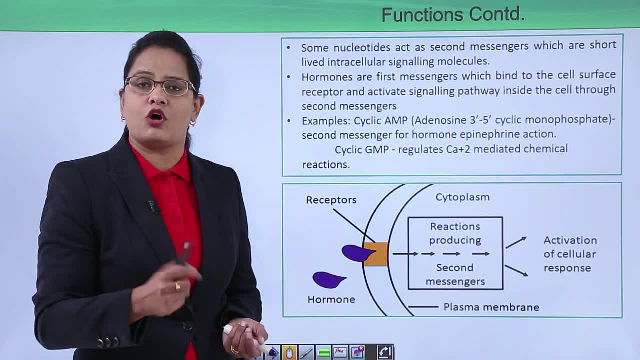 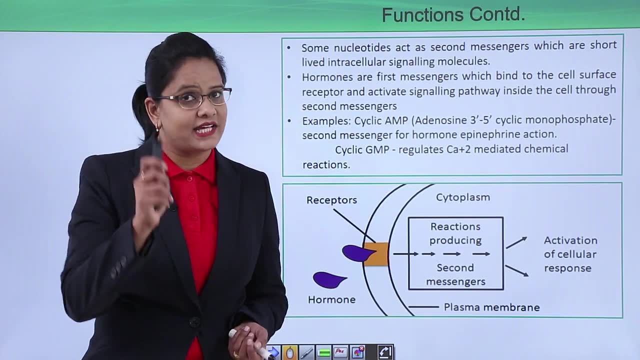 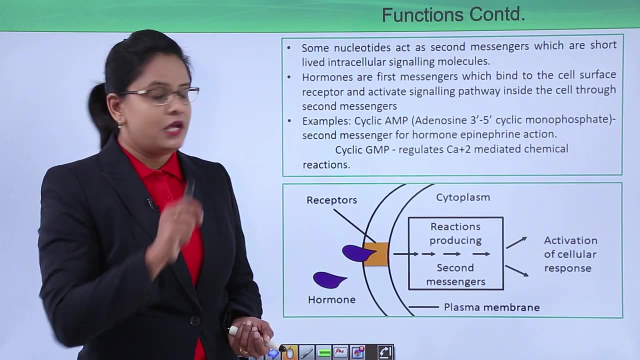 they get activated and a series of reactions goes on which leads to the ultimate cellular function. So the nucleotides act as second messengers. The examples are cyclic inhibitors, which is adenosine 3, prime, 5 prime, cyclic monophosphate. 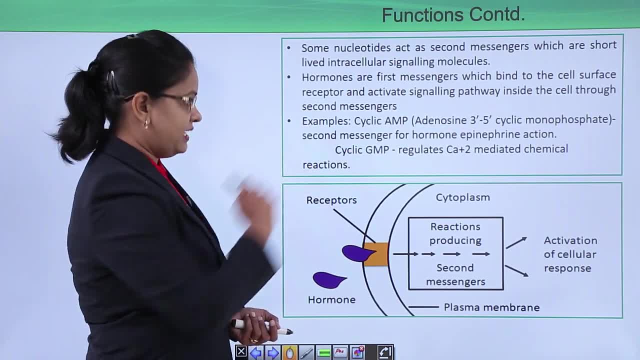 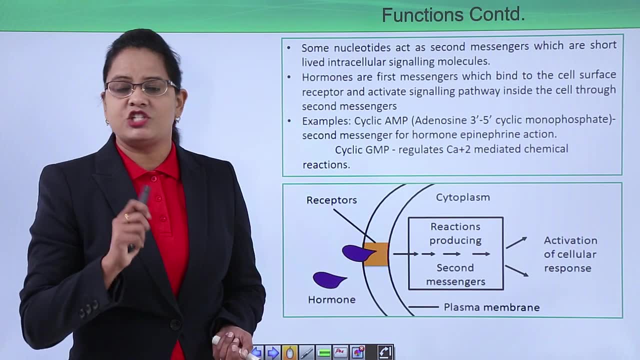 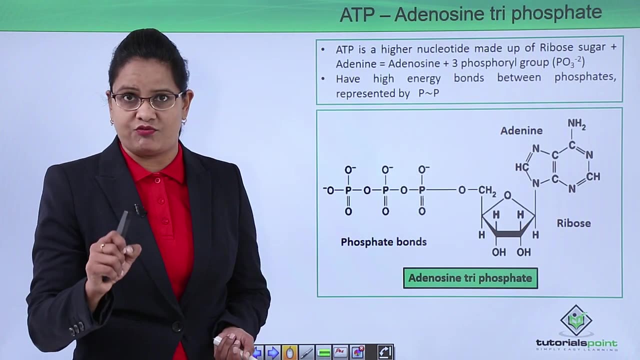 Now this acts as a second messenger for hormone epinephrine and cyclic GMP. This regulates calcium mediated reactions which are present inside the cell. Now the next very important nucleotide, that is, adenosine triphosphate. Now all the energy that we are getting by different reactions like respiration. 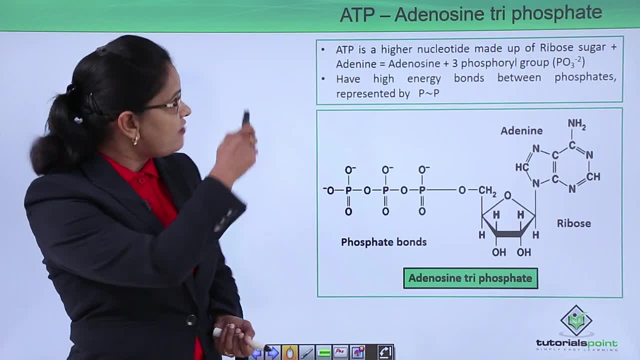 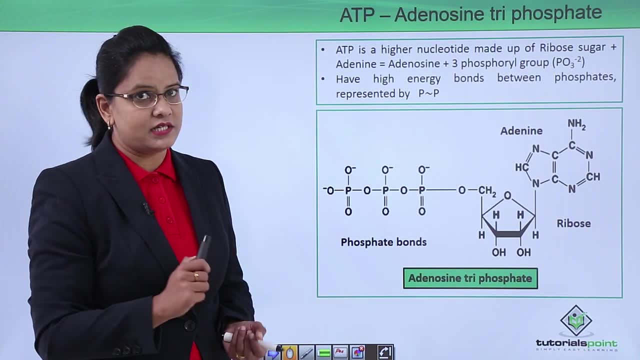 This energy which is produced? it is produced in the form of adenosine triphosphate, So it is a higher nucleotide made up of a ribose sugar. As you can see in the structure, there is a ribose sugar, adenine base and there are three phosphate molecules. 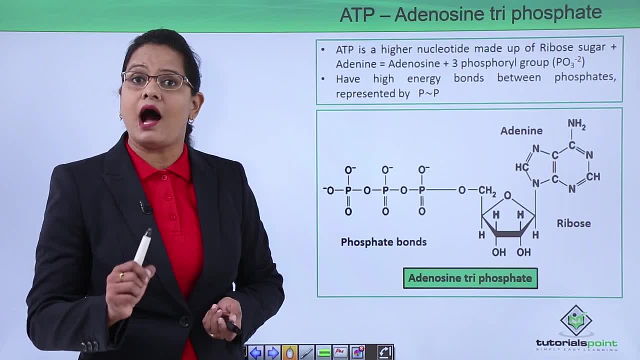 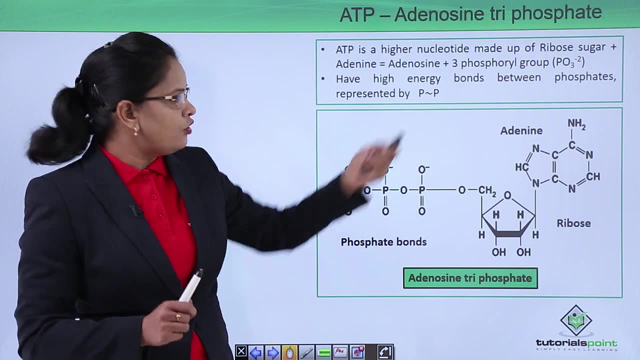 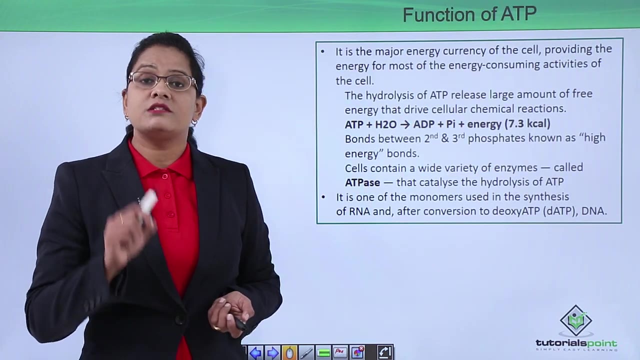 Now, this bond between the phosphate molecules is a very high energy bond, right? Therefore, it is represented by a curved dash. So wherever you see a curved dash, it means it is representing high energy phosphate bonds. Now let us see what is a function of ATP. 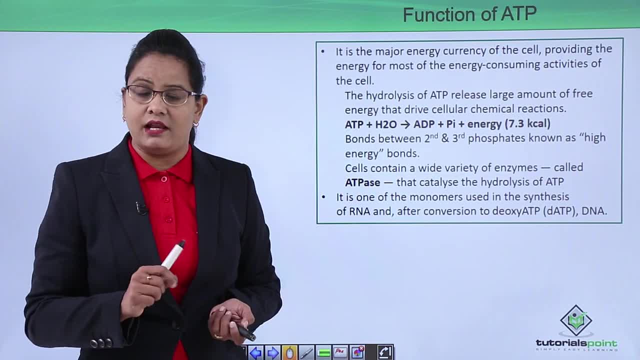 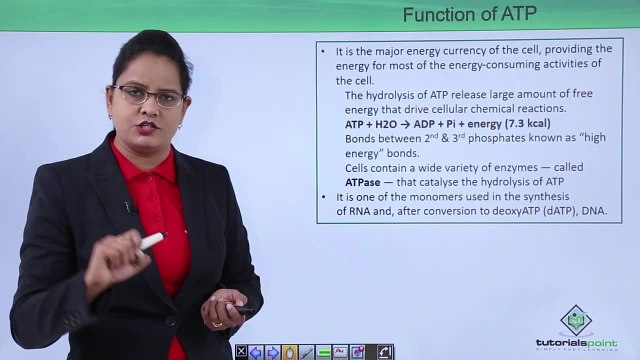 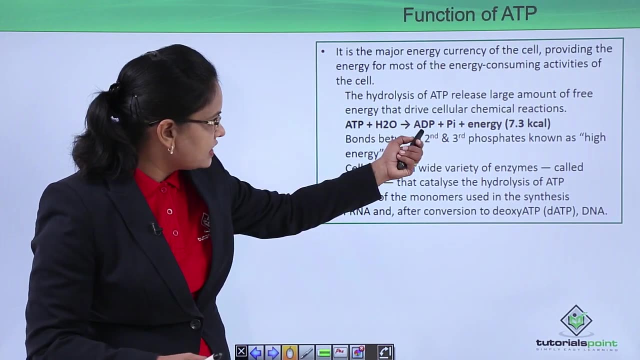 Now, ATP is a major energy currency of the cell. All the reactions in the cell. the energy is produced by adenosine triphosphate. all the energy consuming activities. Now how the energy is produced. This ATP gets hydrolyzed into adenosine diphosphate and a phosphate molecule is released. 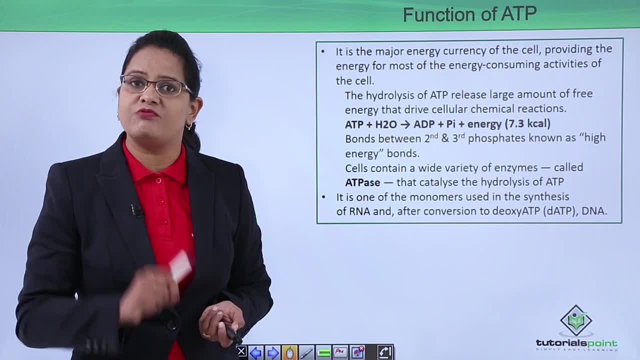 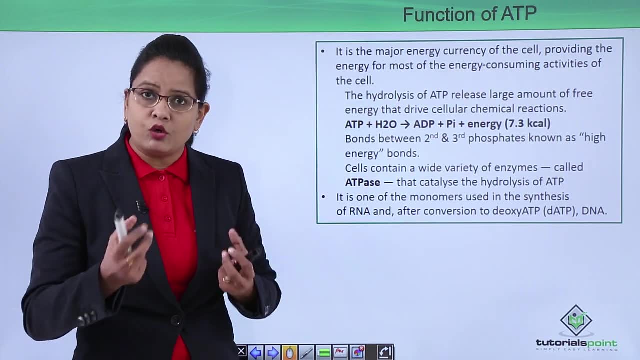 along with the ATP. Now this energy has an approximate value of 7.3 kilocalories, So this is a very large energy as compared to what is our requirement. The bond between second and third phosphate is high energy bond. we have already discussed it. 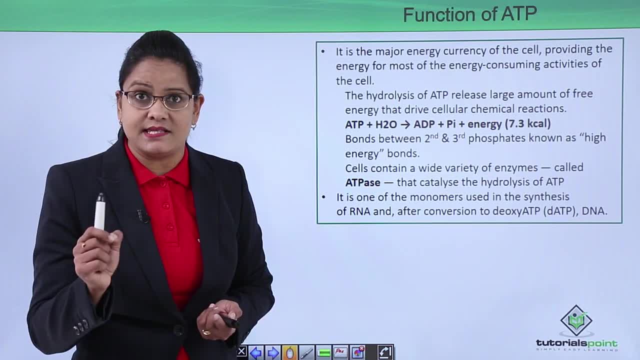 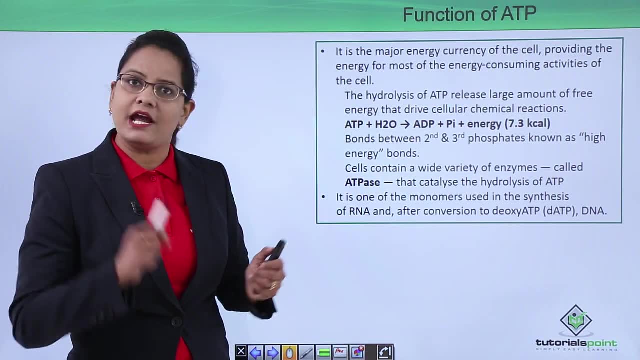 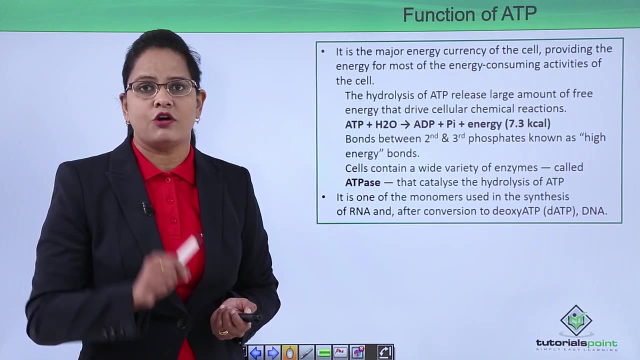 Now there is an enzyme called ATPase. This is the enzyme which, along with water, leads to breaking of ATP into ADP and PI and formation of energy. Another important reason is that ATPase is a very high energy molecule. Another important role of ATP is that it is also a monomer for formation of RNA and DNA. 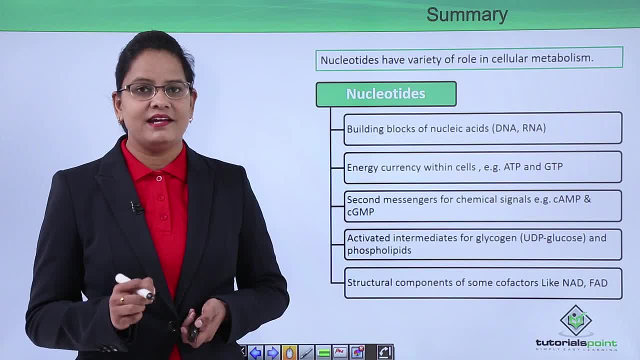 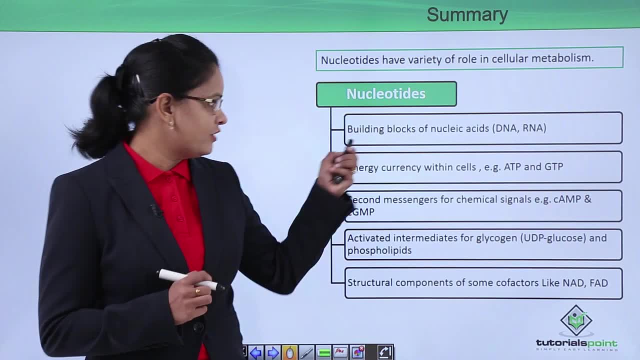 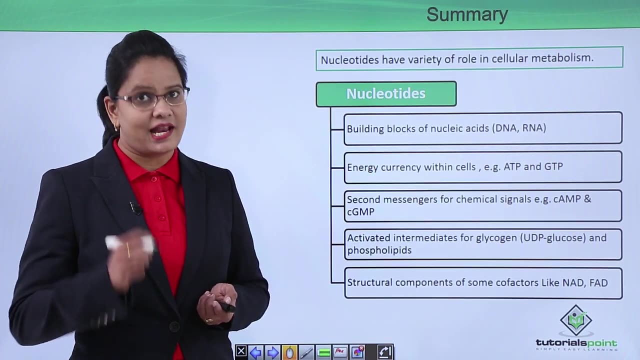 Thus, to summarize, we can say that nucleotides play very important biological functions in a cell. These functions are: first, they act as building blocks of nucleic acids like RNA and DNA. They are the energy currency within the cells, like ATP. 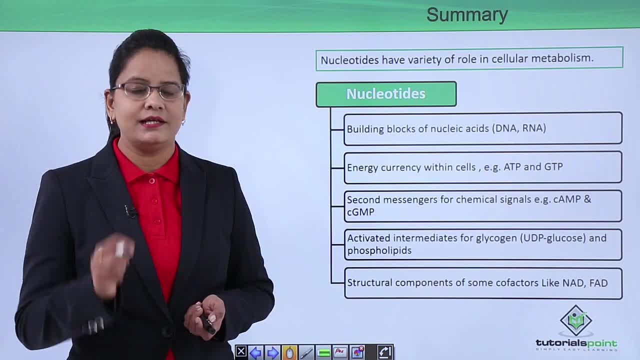